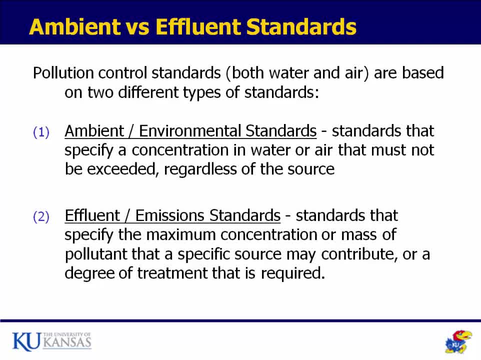 be exceeded, regardless of the source. The idea is that we should be able to go anywhere inside the United States of America and encounter water and air that has a base quality to it. The second type of standard is just is described as an effluent or an emissions standard. 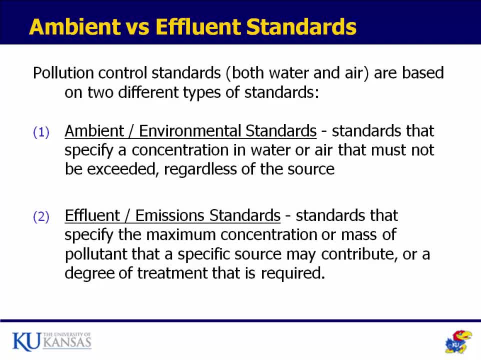 or surface water pollution control standard. This standard is considered as a water pollution control standard. This standard is considered as a water pollution control standard. This standard is sometimes a discharge standard. This is the standard or the maximum concentration or mass pollution that a specific source can contribute. Sometimes the standard is not discussed as a 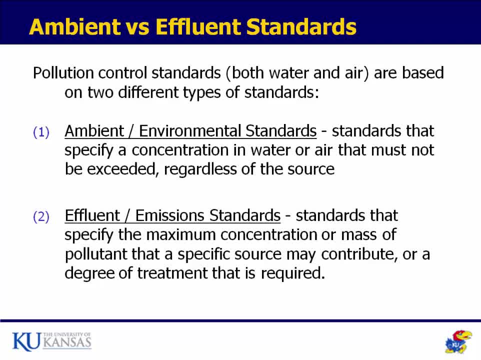 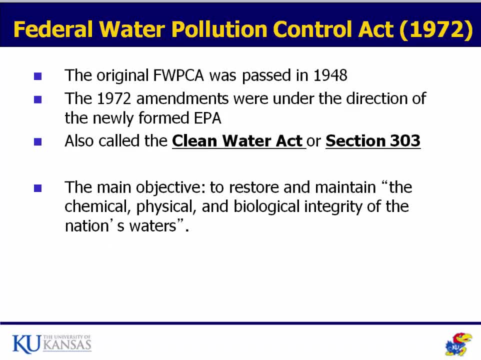 numeric criteria, but rather a degree of treatment that is required. The Clean Water Act's official name is the Federal Water Pollution Control Act. Although it was first passed in 1948, its current form began in 1972 after the EPA was established and amendments were made. This 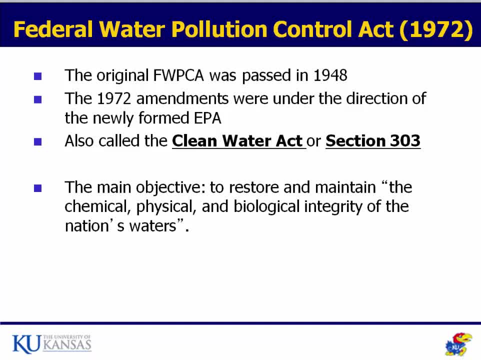 legislation is commonly known as the Clean Water Act or Section 303.. Literally, Section 303 of the Federal Code is where the Clean Water Act is written. The main objective is to restore and maintain the chemical, physical and biological integrity of the nation's waters. The Clean Water. 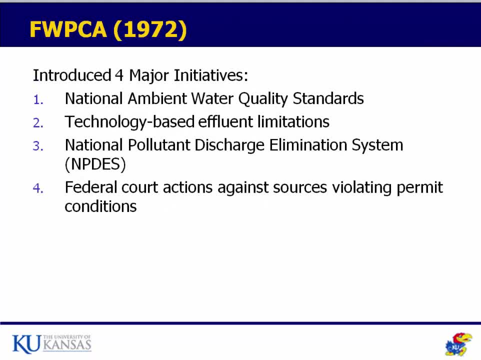 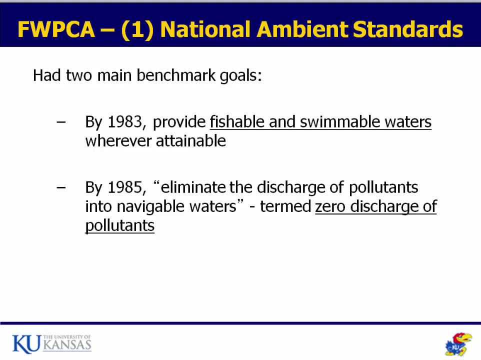 Act, or the FWPCA, includes four major initiatives. We'll go through each of these in brief. For National Ambient Standards, there are two major goals. The first is to provide fishable and swimmable waters wherever these are attainable. Again, this covers both the ecological and the human health. The second was to provide or 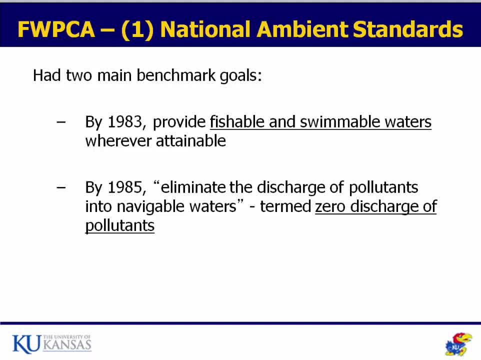 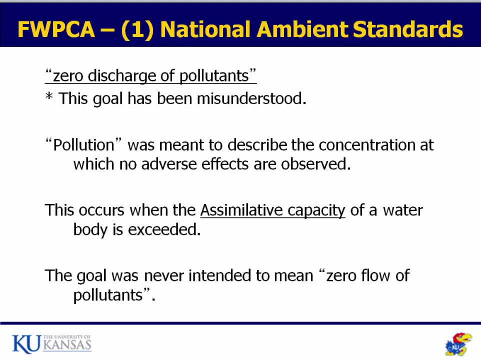 to eliminate the discharge of pollutions into navigable waters. This has been termed the Zero Discharge of Pollutants. Pollution in this case was not meant to mean flow, but rather to describe the concentration at which no adverse effects are observed And no. 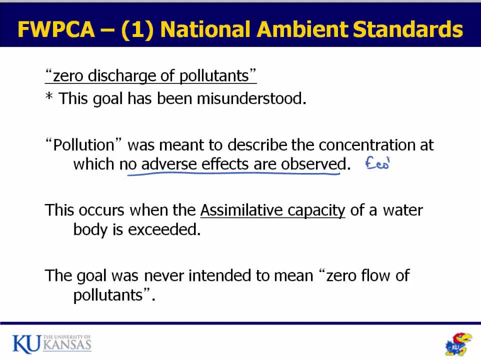 adverse effects include both ecological effects and human health effects. No adverse effects occur when pollution is discharged to a waterbody below the assimilative capacity of the waterbody. Any given waterbody can assimilate pollution or pollutant load and have zero impact. 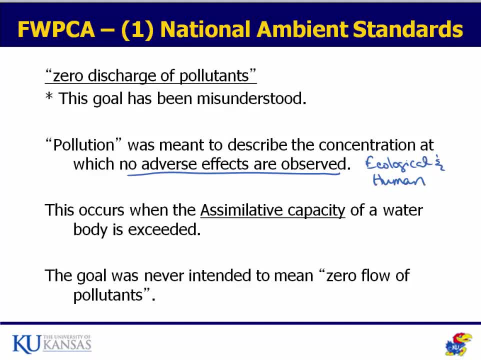 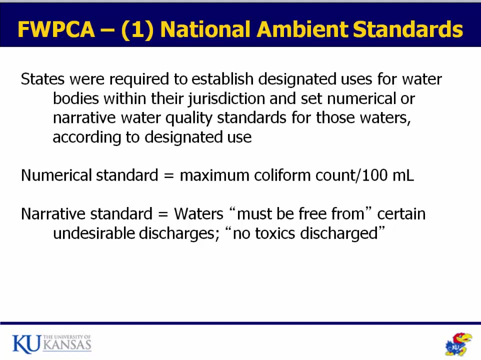 And that zero impact was what this language was intended to be. It was never intended to be zero flow, but rather zero pollution or zero negative effect. This language has been clarified and in amendments a new term has been used, called anti-degradation. Okay, so states were required to establish designated uses for water bodies within their jurisdictions and set either numerical or 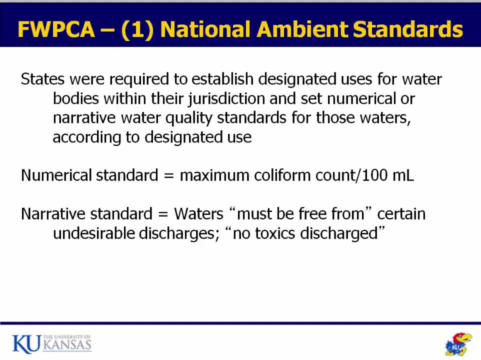 narrative water quality standards for those waters according to the designated use. Examples of numerical criteria for pathogens would be that a maximum coliform count, and that would be written in a number of MPN or number of CFU, are allowed for 100 ml of sustainable. 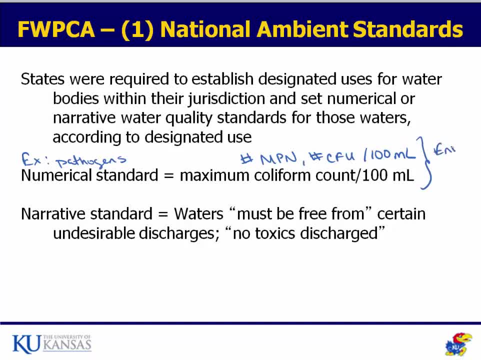 of volume. We will return to this in the environmental microbiology lesson plan that is next, But the numerical criteria is a concentration that should not be exceeded. A narrative standard may be written, such as waters must be free from certain undesirable discharges, or quote: 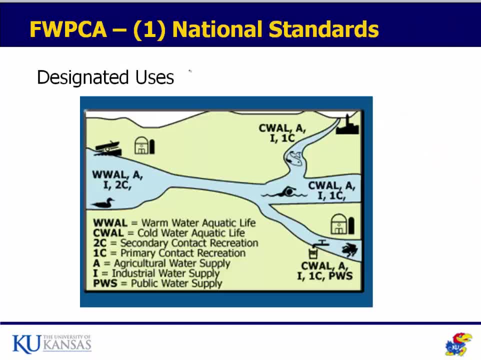 no toxics should be discharged. It's important for states to establish designated uses because water quality standards will vary for the designated use And this is because risk varies with use. For instance, in this river, with several tributaries in one section of the river, you have 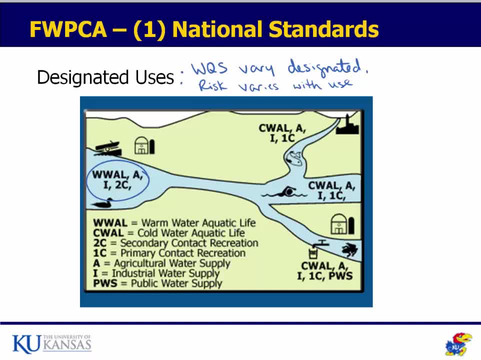 four uses that have been defined: Warm water, aquatic life, WWAL, agricultural water supply, industrial water supply and secondary contact recreation. This would include boating. In this part of the river, though, you have primary contact recreation, which includes swimming, And then, if you look down here at this, 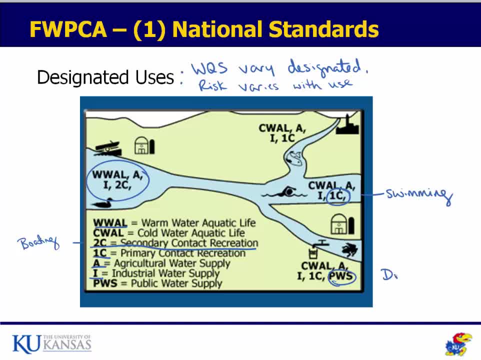 third example: you have a public water supply and so you have drinking water. With each of these uses, you have different routes of exposure and therefore different risk. So when a state sets water quality standards, they set them according to use, which gives you the relationship. 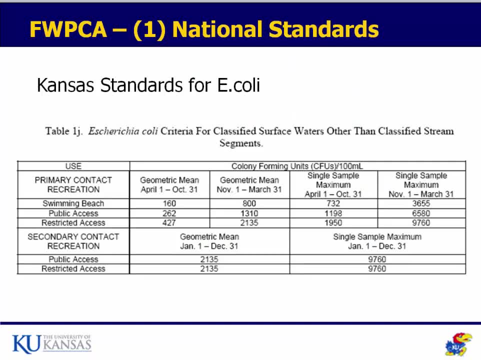 to exposure frequency and duration. Let's look at the Kansas standards for E coli. E coli is the measure of pathogens, or pathogen indicators. Here you have the use according to primary contact recreation and secondary contact recreation, And you have Colony farming. 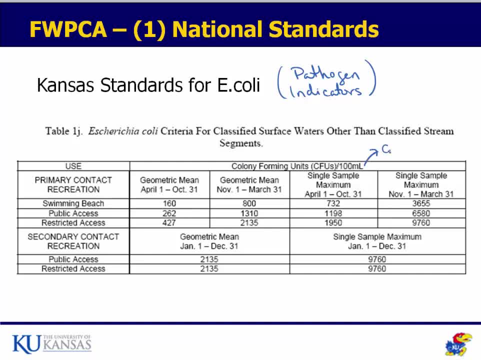 unit per 100 ml. This is the concentration term of E coli For each of the uses. you have, both a seasonal- April to October and November to March- concentration that varies- and then by use For class. I've asked you to print the table of numeric criteria and bring it. 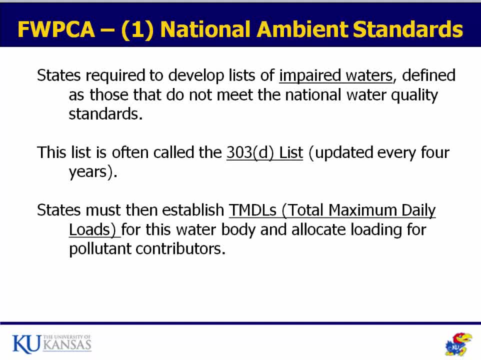 so that we can discuss certain aspects of this more in depth Now. in the Clean Water Act, if a national water body has been sampled and it's found that the concentration of any constituent is higher than the water quality standard, then the state is required to list the water body as: 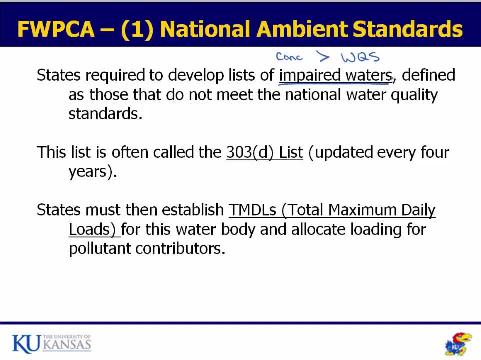 impaired. Impaired waters are defined as those that do not meet the national water quality standard. The list of impaired water bodies is officially referred to as the 303d list or section d of 303 of the federal code. It is updated every four years. When a water body is listed, the state. 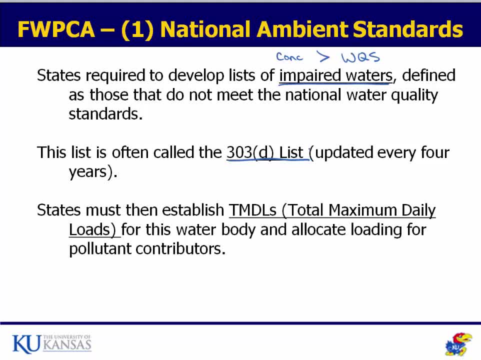 is required to establish total maximum daily loads for that water body. The state has to determine the source of the pollution and then allocate the amount of water that the water body is polluting. The unit for load is mass per time. This process is pretty complicated because simply, 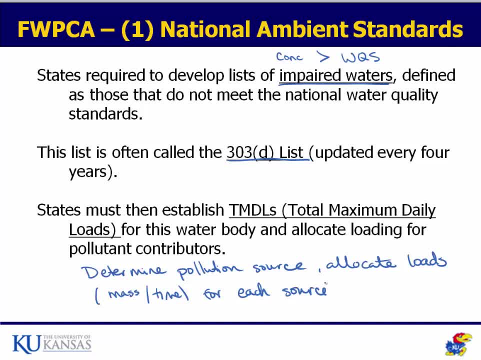 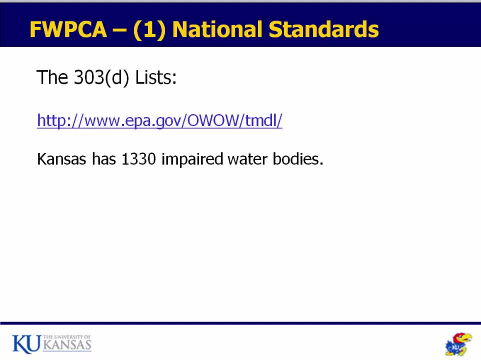 studying all of the sources of pollution can be fairly time intensive In class. we'll go to this website, but you're welcome to go there now too. This is the official list of all of the impaired water bodies in the nation and this changes every four years, but currently Kansas has. 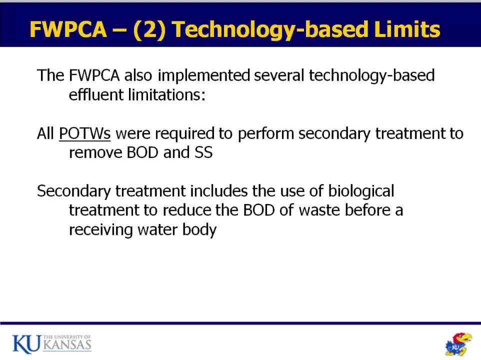 1,330 impaired water bodies in the nation. This is the official list of all of the impaired water bodies in the nation and this changes every four years. but currently Kansas has 1,330 impaired water bodies in the nation and this changes every four years, but currently Kansas has been. 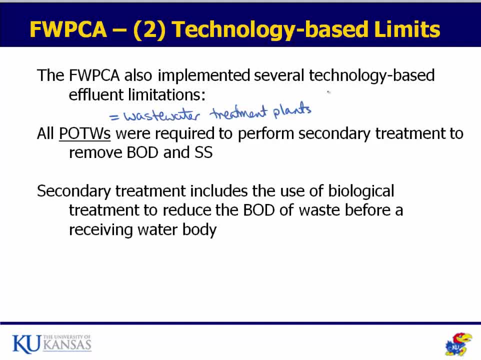 concerned by these, trying to determine the exact names of these impaired water bodies. Move on. So the second of the four major initiatives of the Clean Water Act was to set technology-based effluent limits All publicly owned treatment works, and so POTWs refers to Wastewater Treatment plants. 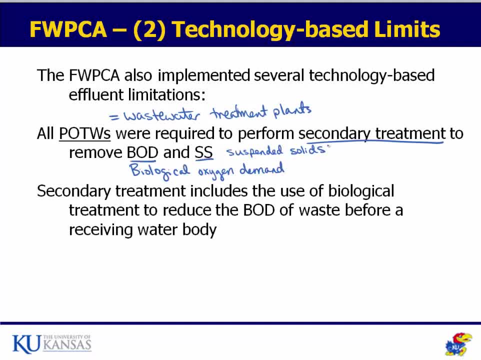 All wastewater treatment plants were required to perform secondary treatment to remove biological oxygen, démand BOD and suspended solids. SS Secondary treatment is defined as the use of biological treatment to reduce BOD of waste before entering a receiving water body In Lesson Plan 9 and 10,. 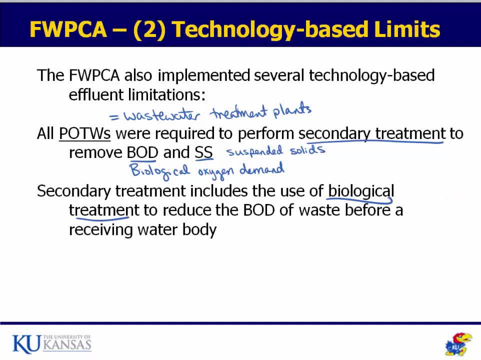 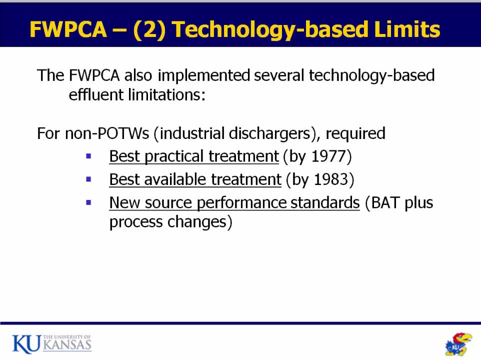 we will be discussing BOD intensively As we move into the discussion of wastewater treatment, you'll learn that biological treatment is the critical step for secondary treatment For non-POTWs or industrial discharges. the Clean Water Act said that the best practical 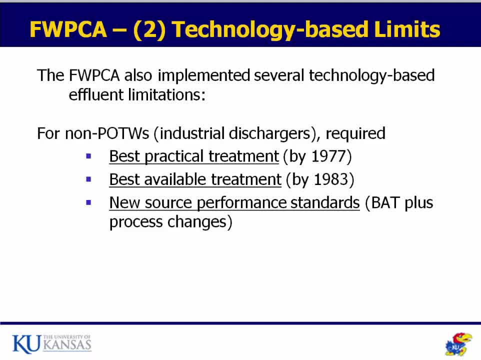 treatment should be instituted by 1977 and that the best available treatment should be instituted by 1983. That was about a decade from when this was first enacted. I will tell you that this was a large burden to industry and was loosened in amendments. The cost analysis was too great. 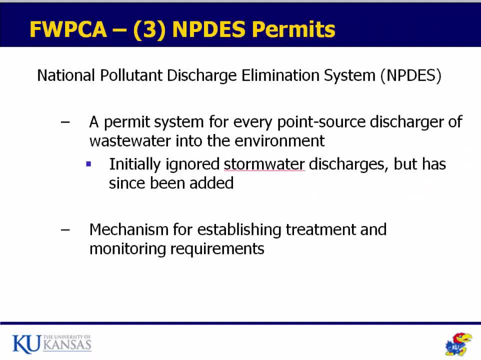 for BAT installation. The third section of the Clean Water Act established the mechanism for BAT installation. The third section of the Clean Water Act established the mechanism for BAT installation. The third section of the Clean Water Act established the mechanism by which effluent standards would be propagated. This is known as the National Pollutant Discharge. 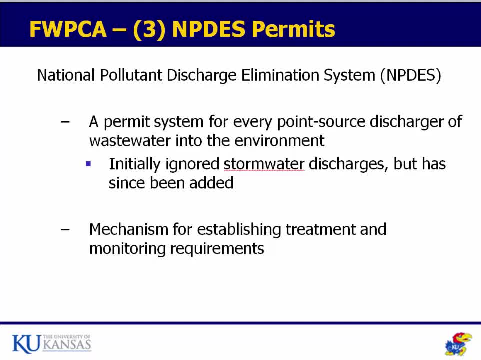 Elimination System, or MPDES. This is a permit system for every point source: discharger of wastewater into the environment. It initially ignored stormwater but that has been added in amendments So currently MPDES follows wastewater and some stormwater. The MPDES permit outlines the 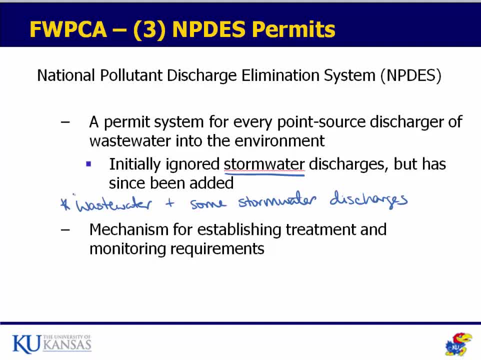 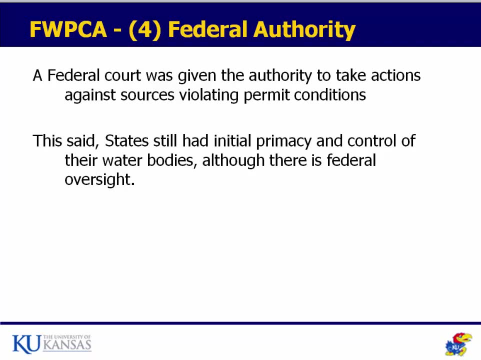 established treatment or required treatment and also the required monitoring that must be reported to the state. You've been asked to read a wastewater treatment MPDES permit and we'll be discussing that in class. The fourth section of the Clean Water Act establishes federal authority That said states hold the initial primacy and control of the water. 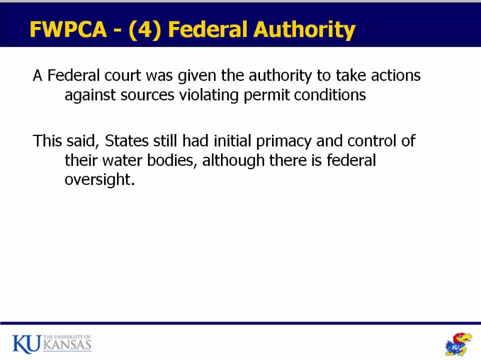 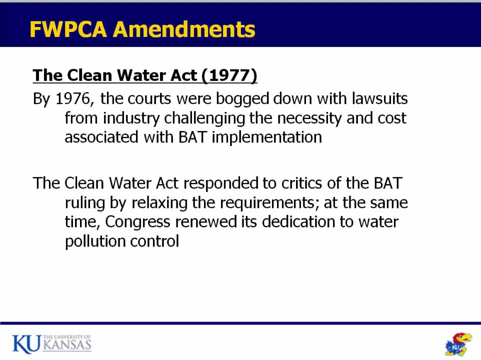 bodies. Federal government is only allowed to step in if the states are not complying, As with all environmental legislation. there have been several amendments that have been passed. In 1976, the courts were bogged down with lawsuits, mainly from industry focused. 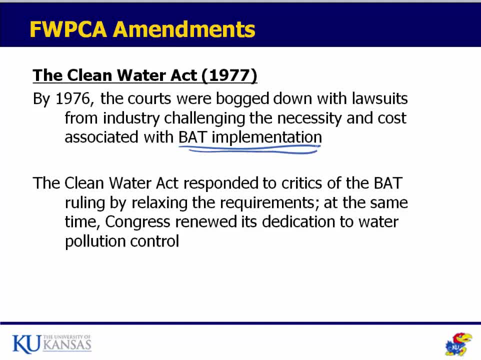 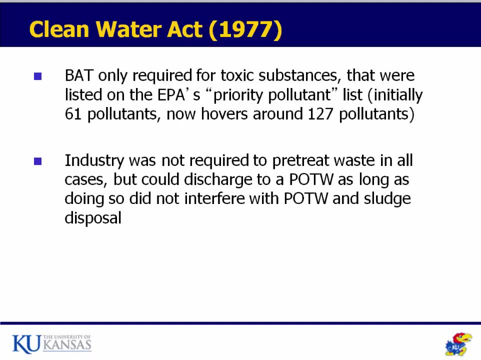 on the BAT requirement that had been put into place. The Congress then renewed the Clean Water Act, but also lessened the requirements for BAT. BAT is currently only required for toxic substances. These are listed on the EPA's priority pollutant list. It was 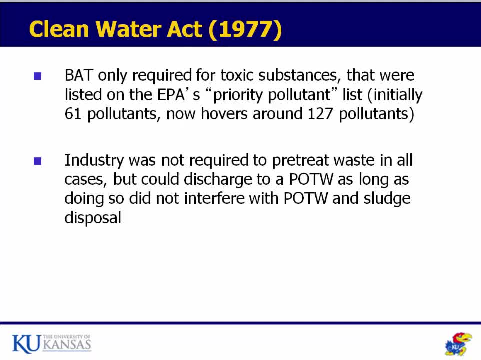 initially 61 pollutants and now hovers around 127.. These are considered the most toxic pollutants and therefore the cost benefit of requiring best available technology is considered acceptable. With this amendment, Congress also said industries were not required to pre-treat waste as long. 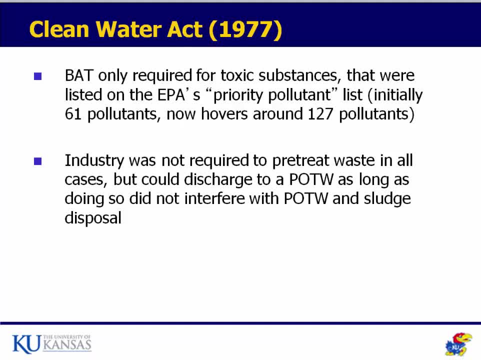 as the publicly on treatment work was willing to take the waste and treat it in the municipal plant. This has been commonly used In the United States as a way to also attract industry to cities. If municipalities are willing to treat waste for you, that is a huge boon to industry. Following with lessening 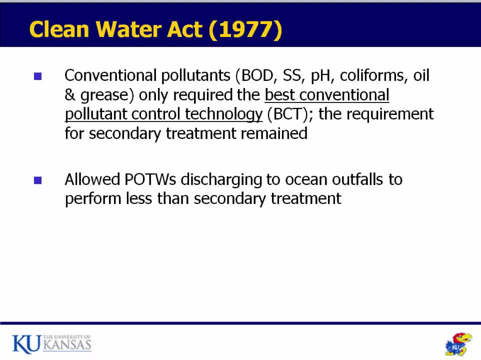 the best available technology requirement. conventional pollutants such as BOD, suspended solids, pH coliforms- Coliforms are a pathogen indicator that we'll discuss in the next lesson, plan Oil and grease. These are considered the conventional pollutants. These only require best conventional pollutant. 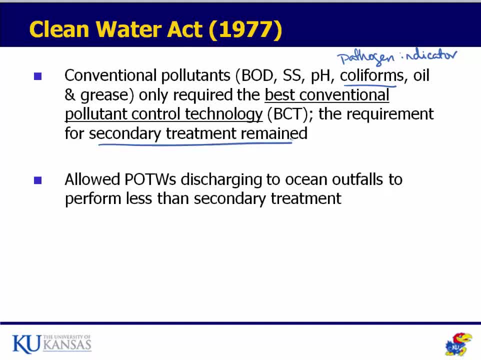 control technology, And that is defined as secondary biological treatment. The exception to this are POTWs that discharge to the ocean. These POTWs may be granted an NPDES permit with lesser treatment required than secondary treatment, And the only logical reason to this is that the assimilative capacity of the ocean is large. This is because of the 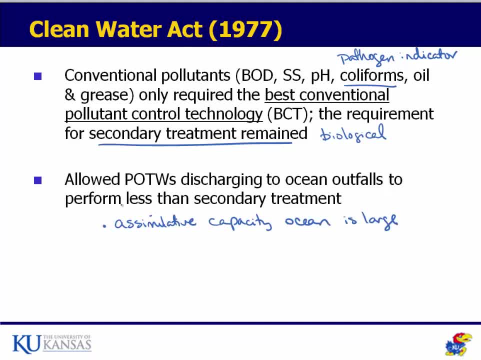 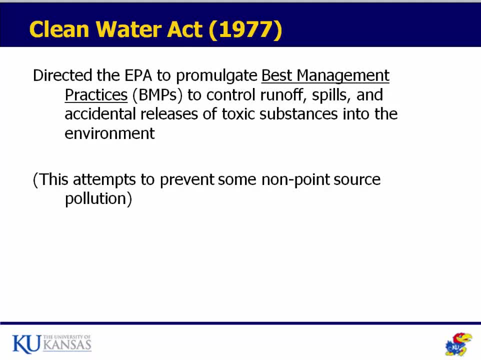 POTW. This is not a given exception to the rule, however, In the 1977 amendment, the EPA was also directed to promulgate best management practices, or BMPs, And BMPs were to control runoff spills and accidental releases of toxic substances into the environment. The 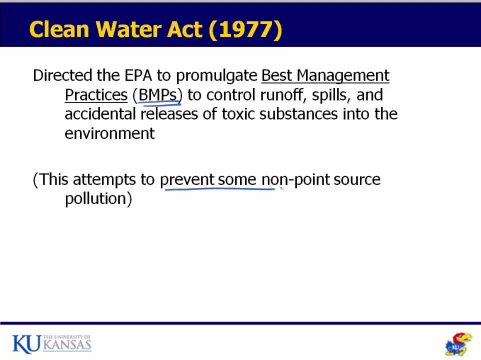 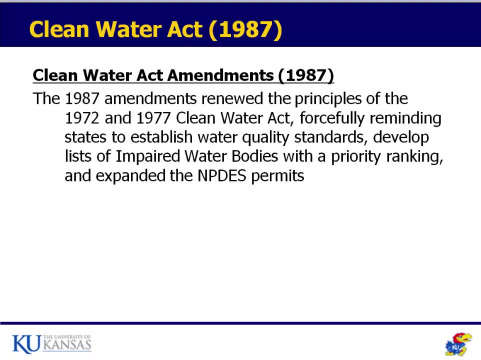 spirit of this was to begin to prevent some non-point source pollution. In 1987, the amendments to the Clean Water Act were renewed And strengthened with respect to the 303 list. because there are so many impaired water bodies, states are now required to issue a priority ranking of the list so that they 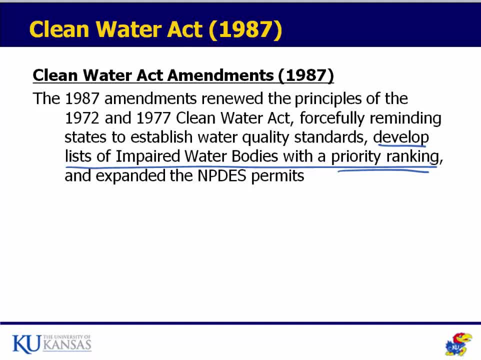 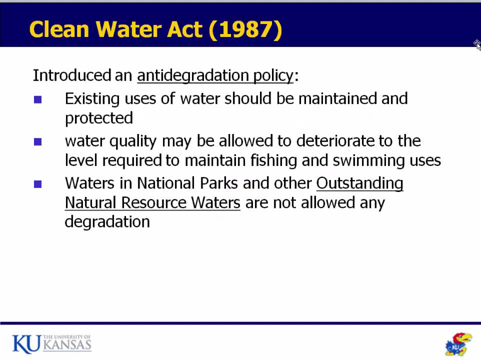 can begin to try to clean up the most polluted water bodies. The second strengthening aspect of this are that the NPDES permits were expanded, specifically with regards to anti-degradation policy and stormwater. The 1987 anti-degradation policy states that existing uses of water should be maintained. 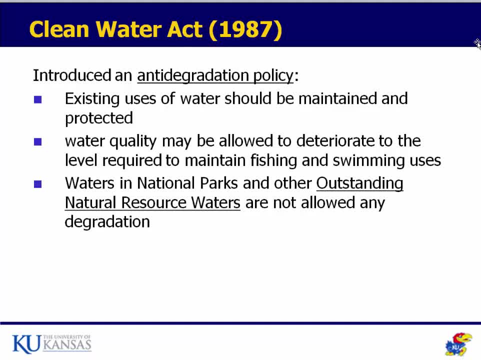 and protected. However, within the original use that was determined, water quality may deteriorate to a level that still maintains that use. This 1987 amendment also defined outstanding natural resource waters. We won't go into this aspect of the rule, but we will go into this aspect of the rule. 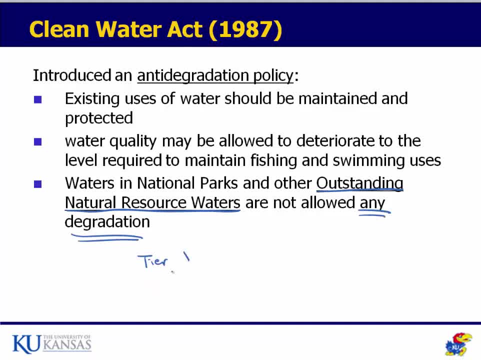 too much. But I will say that there are Tier 1 waters, Tier 2 waters and Tier 3 waters, And the Clean Water Act now says that there is some degradation that is allowed for each of these, But the highest level of maintenance or zero anti-degradation that is allowed. 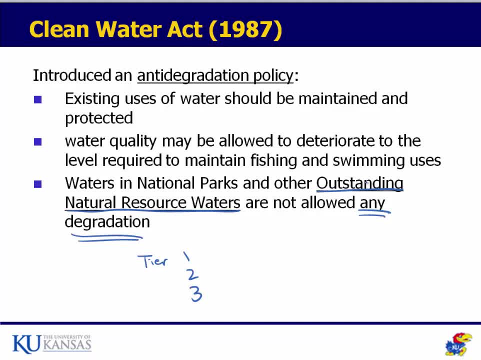 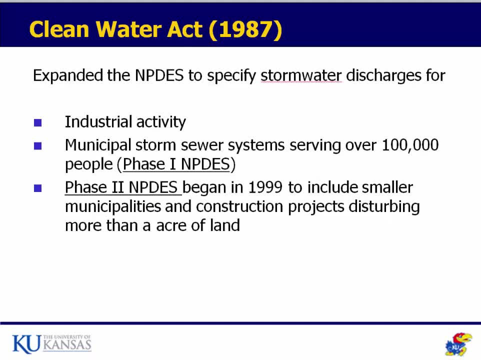 is for national park waters and any other water body that has been determined as an outstanding natural resource water. The last part of the Clean Water Act that has been passed is the expansion of the NPDES permit. NPDES permits were already required for any industry or publicly owned treatment work or any point source discharger Phase. 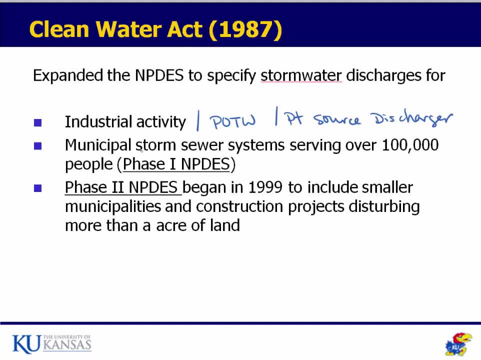 1, NPDES also expanded this to include any municipal storm sewer system that serves over 100,000 people. Prior to this, stormwater systems that were not combined with sewer systems can overflow directly to receiving water bodies without any discharge criteria, And in 1999, Phase 2 began, which said that any smaller municipality should begin to have 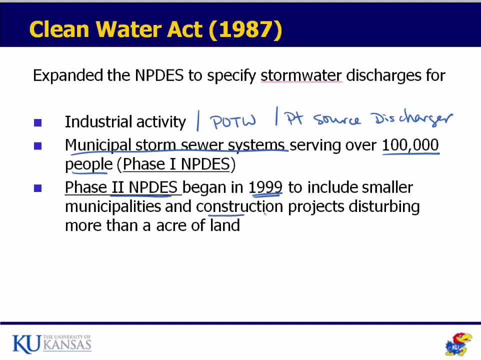 an NPDES permit for their stormwater and construction projects more than one acre, And so this really intersects with construction management, And you should understand that construction sites are now considered point source dischargers under this ruling. Although Phase 2 has been in the register,